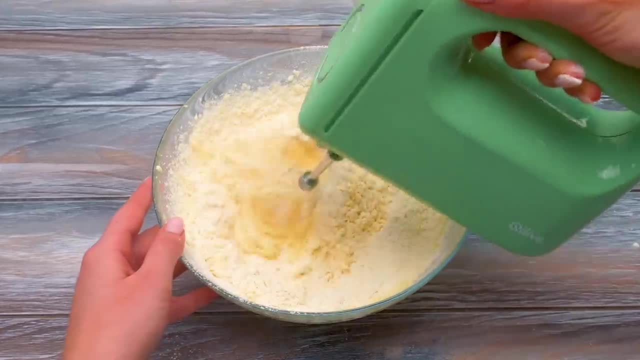 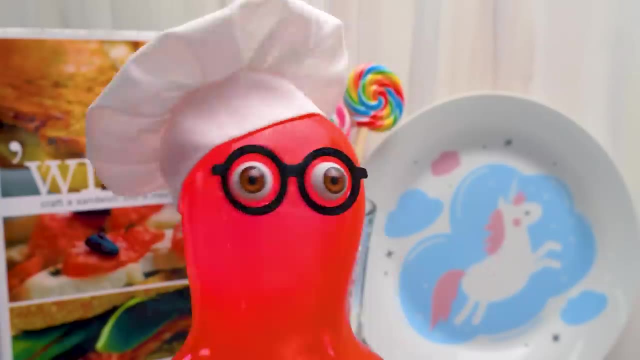 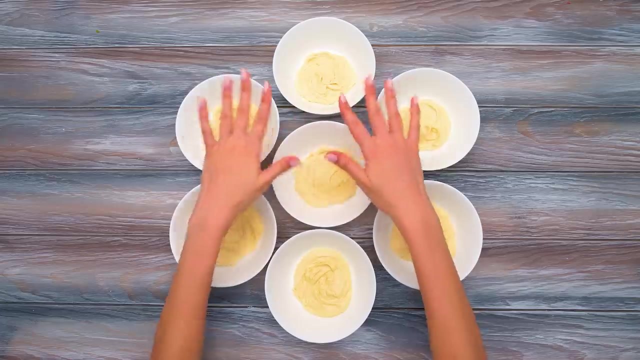 And now let's mix it all well. Mamma mia, It's gonna be the best batter ever. Now guys wanna see some magic. You may ask why we need so many bowls with the batter, And I'll tell you that we're making a very unusual batter. 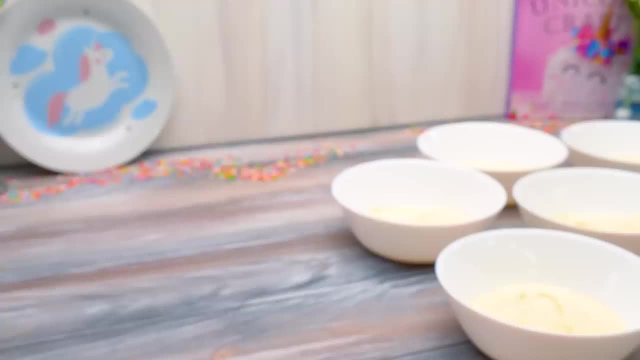 And I'll tell you that we're making a very unusual batter. And I'll tell you that we're making a very unusual batter. We'll see which one will be the best one this time. We'll see which one will be the best color and, of course, we're adding much före picked. 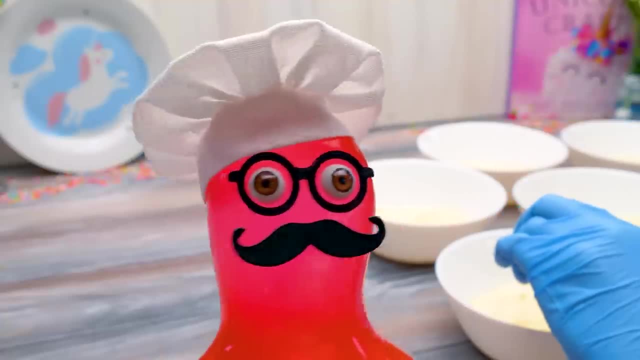 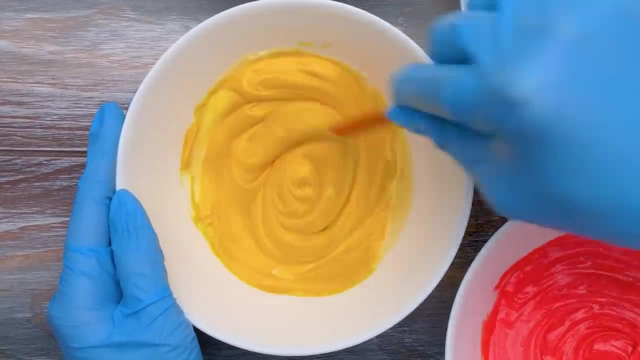 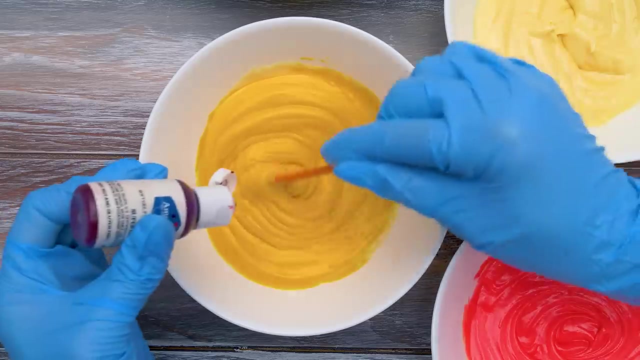 It will be made up of many colorful, delicious cupcakes. Uhh… hey, Siwa, I don't get it. is this yellow or orange Sammy? this batter is gonna be orange Sammy, this batter is going to be orange. 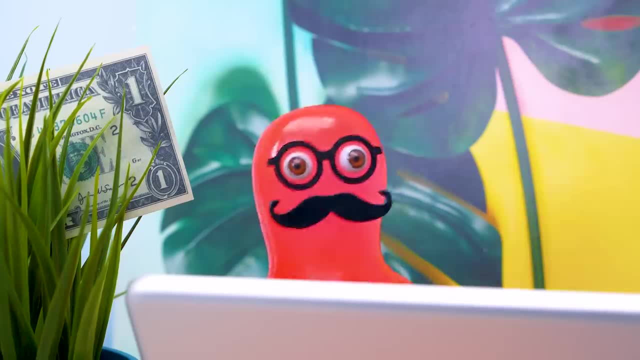 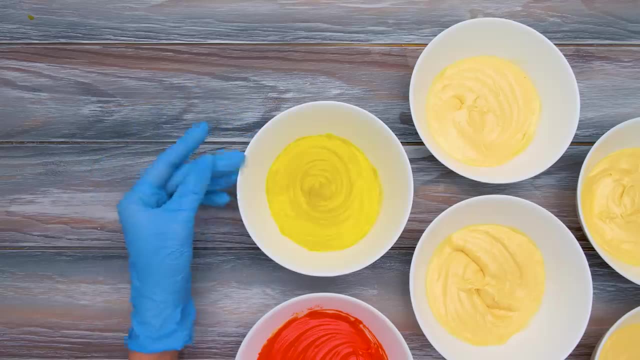 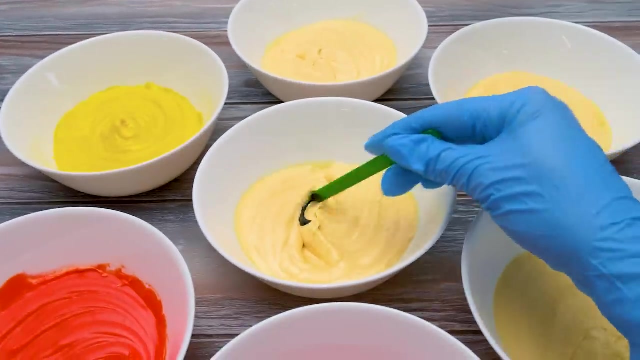 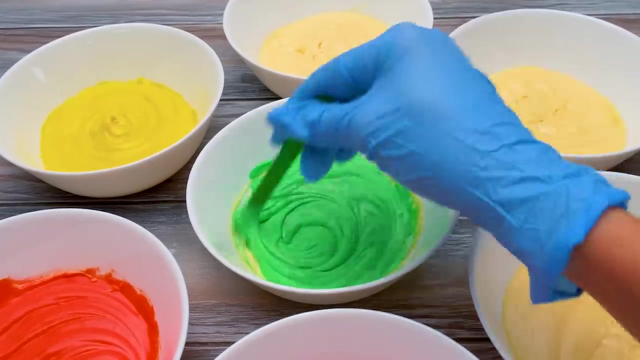 See, The sale of unicorn glitter is lower than last year. How come? I suppose we need to use some unicorn magic. Ah, so beautiful. We need to change our rainbow coloring strategy. Rainbow coloring strategy Sounds um unusual. It seems like these seven colors are out of next year's trends. 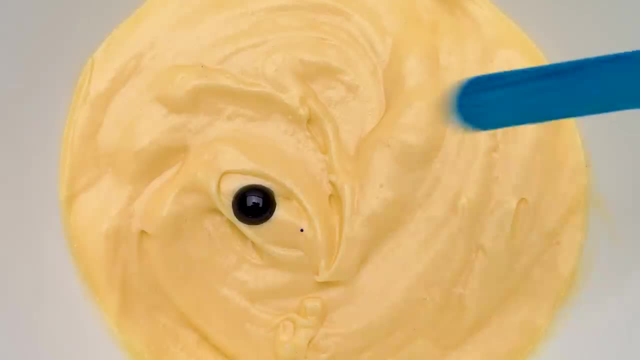 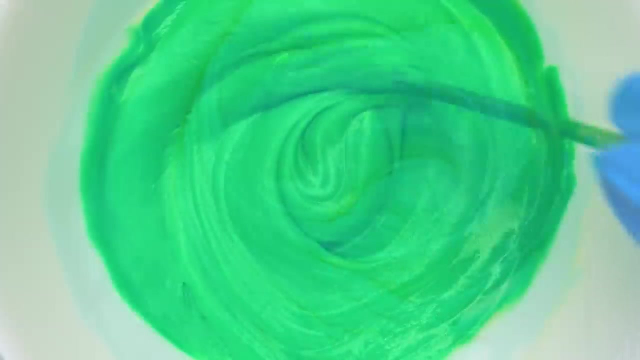 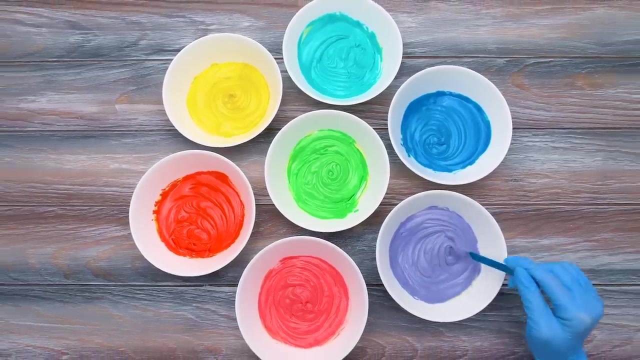 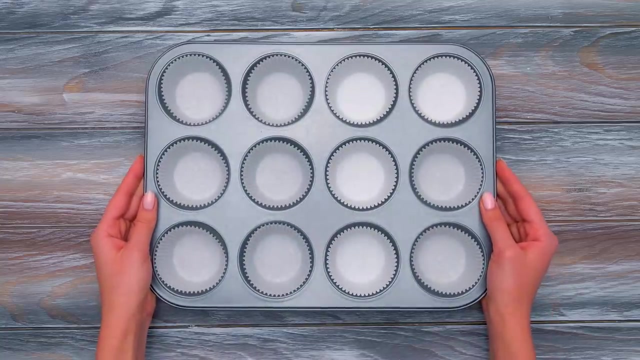 Don't worry, Sammy, Unicorns and rainbows will always be relevant, But still, what was your meeting all about, Sam? So it's our unicorn business. you know Your most important business is helping me with craft. Oh guys, everything turned out so great. 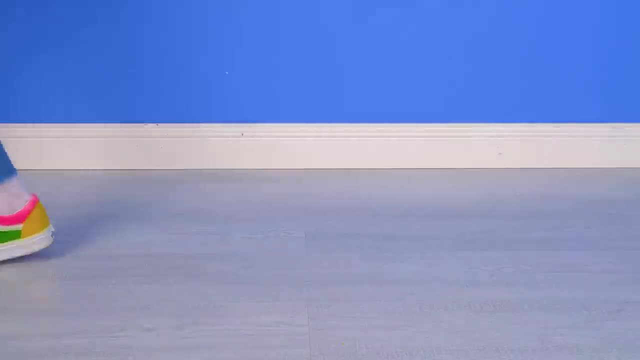 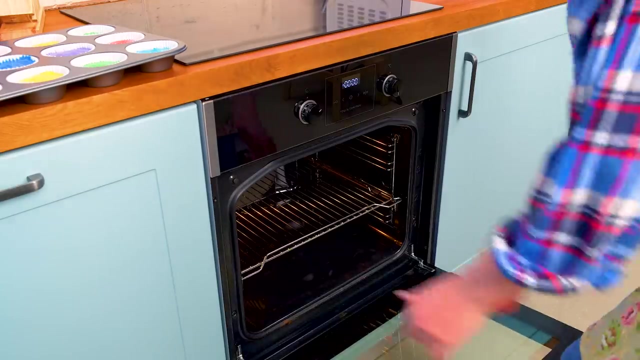 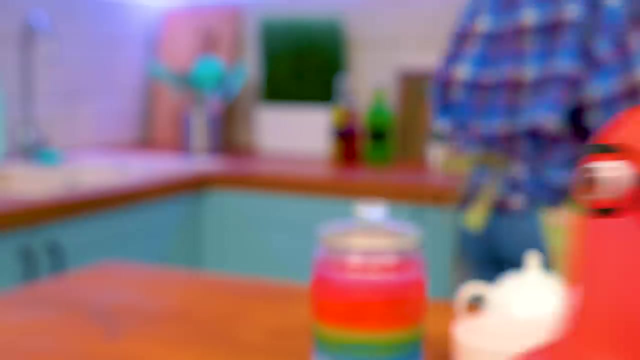 Now let's put the cupcakes into the oven. Guys, we should bake our cupcakes at 190 degrees Celsius. Exactly This temperature is perfect for this batter. Guys, ask an adult to help you, because the oven is really hot. Bake the cakes for 20 to 25 minutes and keep an eye on them. 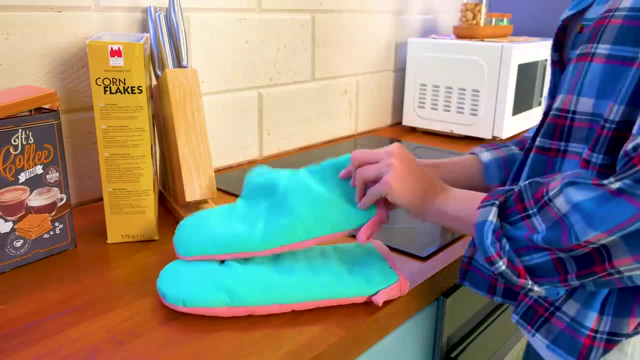 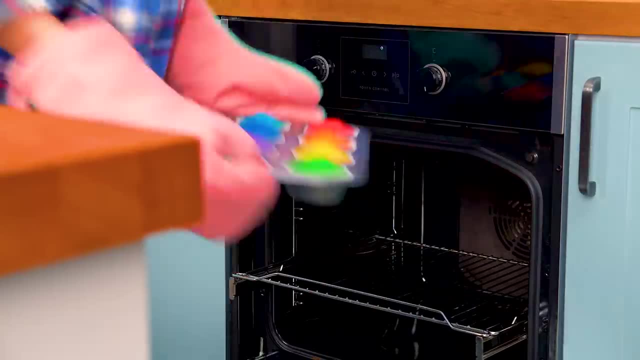 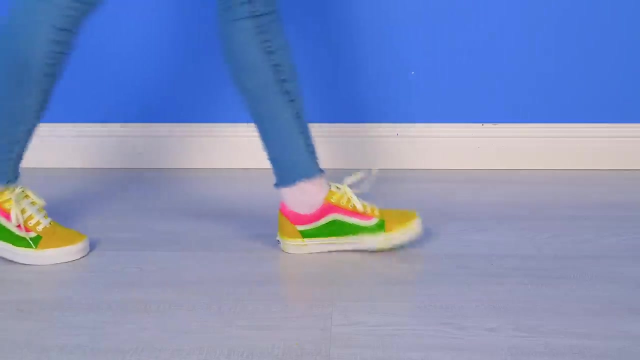 Oh, everything is ready. Don't forget to use oven gloves so you don't burn yourself. Now let's take the cupcakes out of the oven Up. Mmm smells terrific. Da-da-da-da, da-da-da, da-da-da. 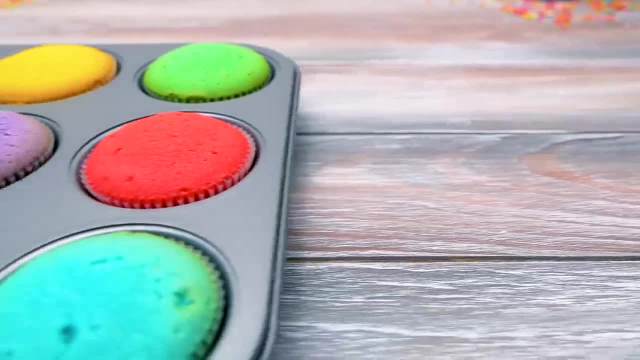 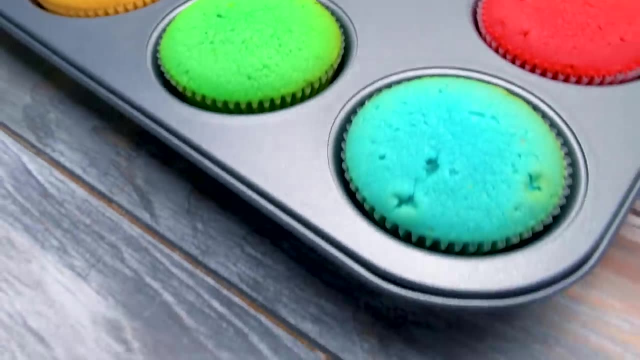 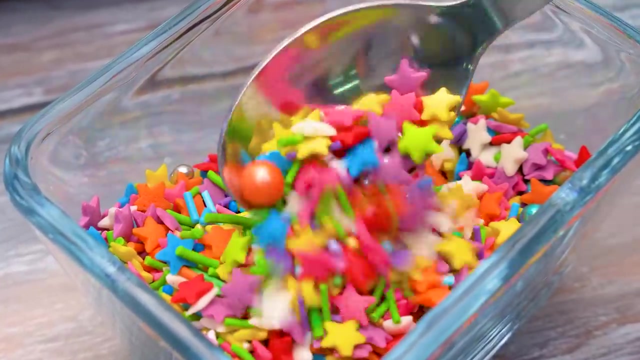 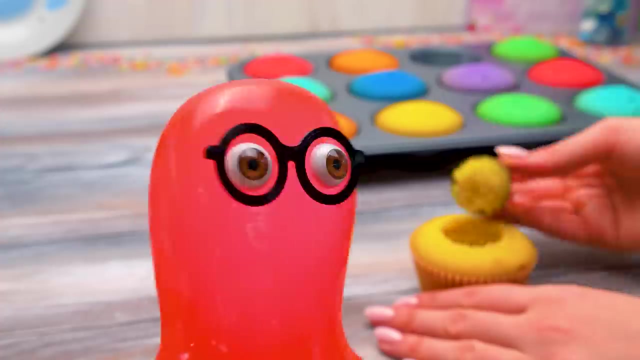 Here are our cuties. It looks so yummy, Yay, Wow, that's a real unicorn Miracle. I think you'll be happy to know that the filling is also in a unicorn style, So we can relax. Vogue says that old rainbow colors will be on trend for the next five years. 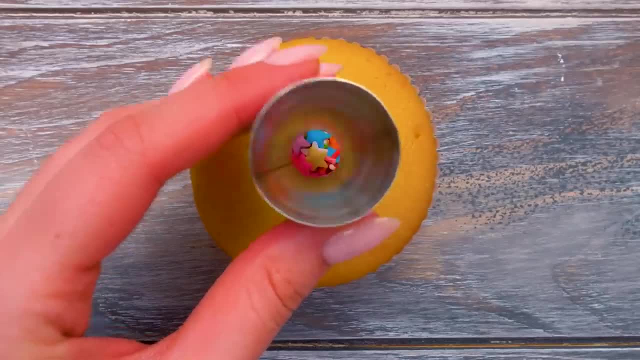 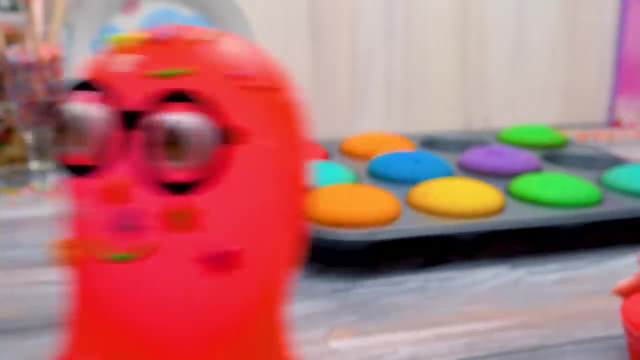 That's great. Then we can fill our cupcakes with these tasty sprinkles. I hope Sammy hasn't eaten all of it. Hey guys, I've rebranded myself So fancy, isn't it? Very stylish. By the way, I'm really happy that you're not so big and didn't eat a lot of the sprinkles. 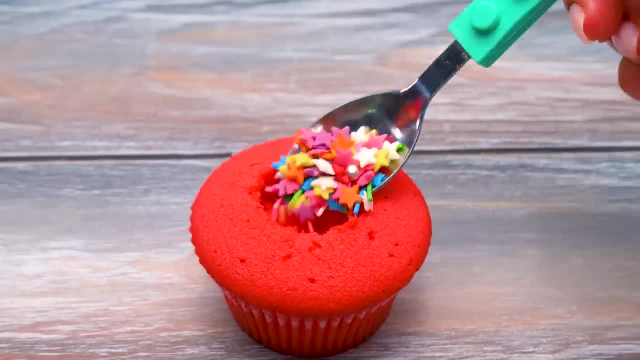 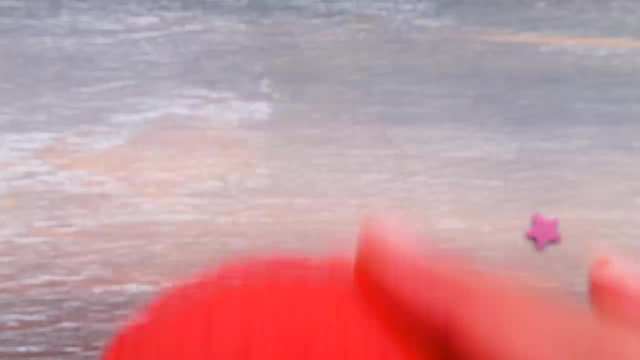 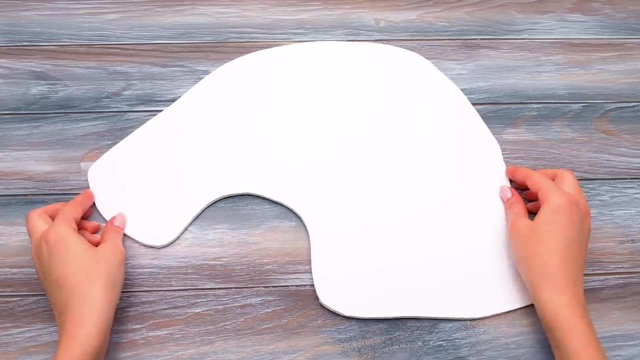 There's enough to fill all of our cupcakes There A little bit more And close it This way. Guys, if you like our cakes, give a thumbs up and subscribe to our channel. By the way, maybe you should write a book about your unicorn business. 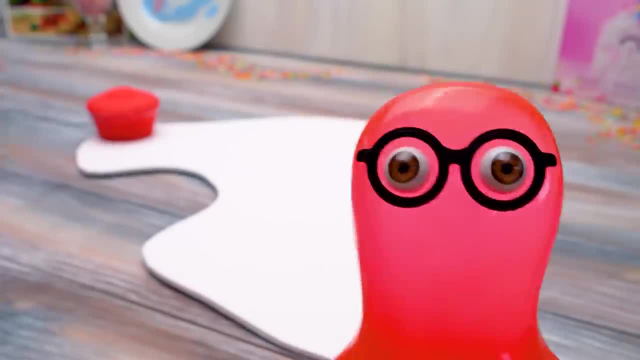 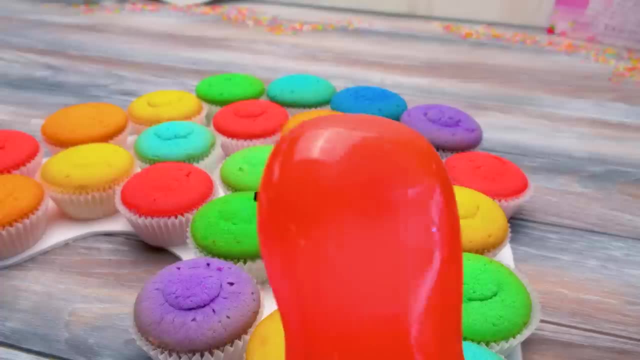 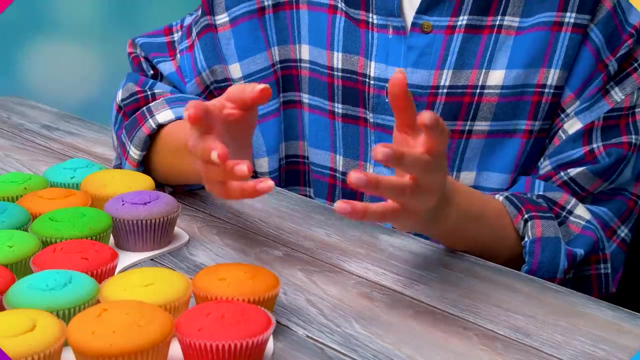 Oh, nice idea, Something like My Way to the Unicorn Success. Guys, check out our unicorn Sue. it doesn't actually look like one. Give me several minutes and you'll see what I'm talking about. Guys, I've got something really cool for you. 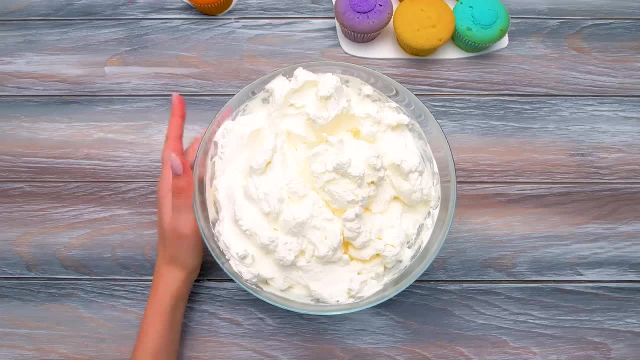 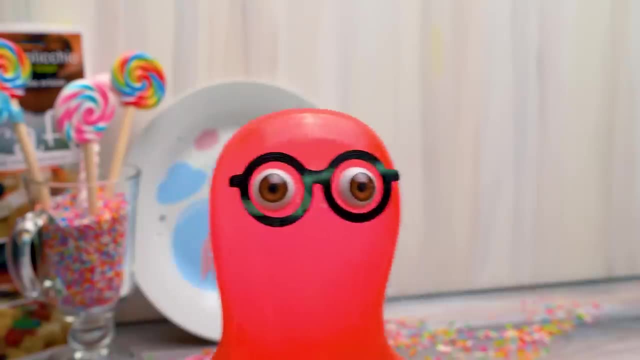 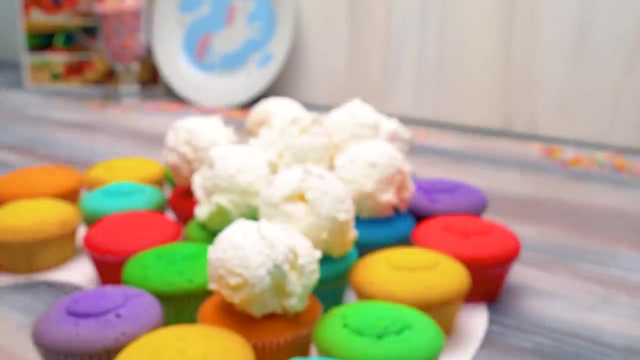 Check out this fluffy frosting. Doesn't it look like a unicorn cloud? Voila, Oh, this buttercream frosting looks so yummy. Sue, can I taste it? Please, Please, Just a little bit, Sammy. Oh, how I love stealing a bite while you're cooking. 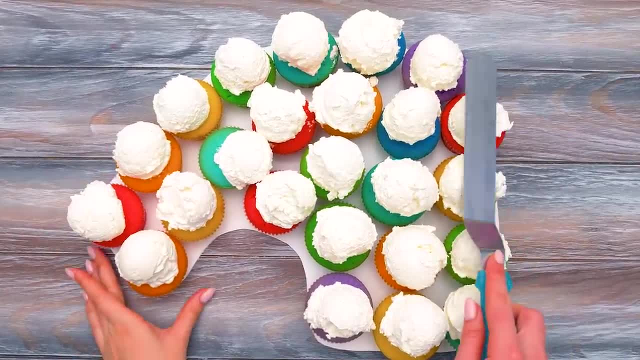 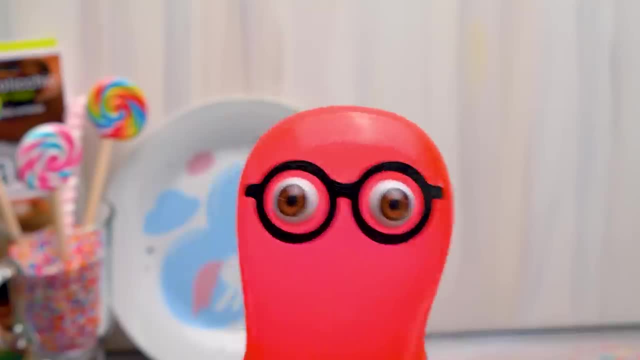 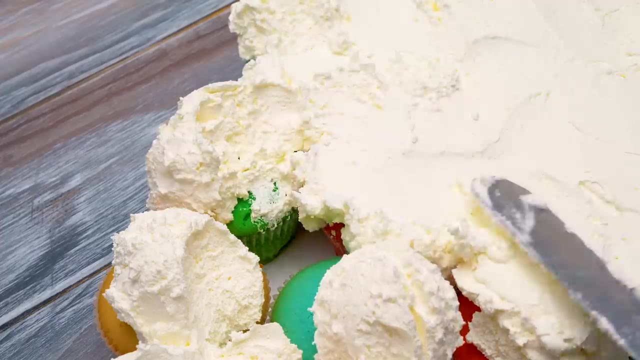 Now we need to evenly spread the frosting. Guys, be careful not to eat everything before the final result. Sammy, calm down. When I look at this delicious frosting-covered cake, I can think of nothing else. I totally agree. Awesome Guys. give a thumbs up if you like how the cake turned out so far. 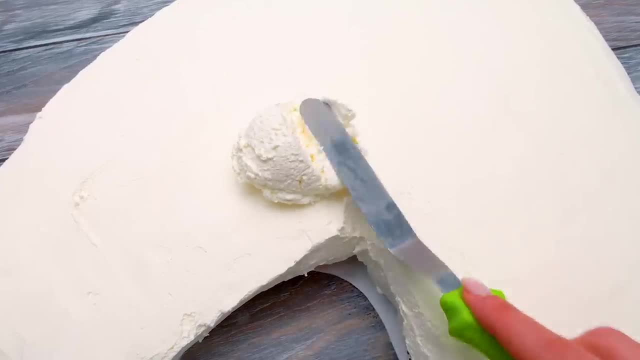 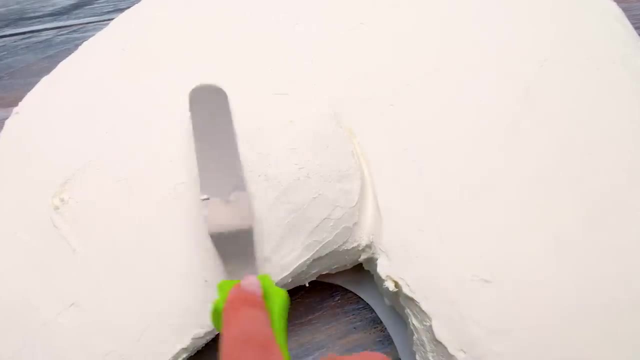 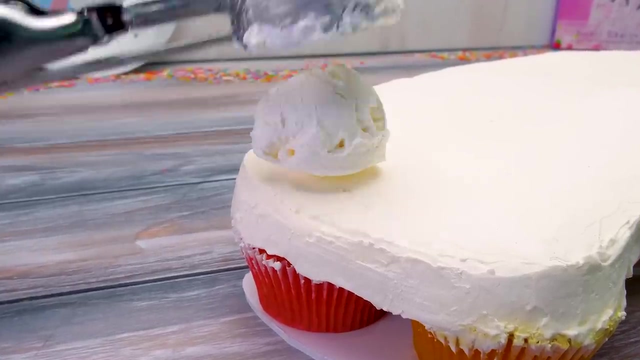 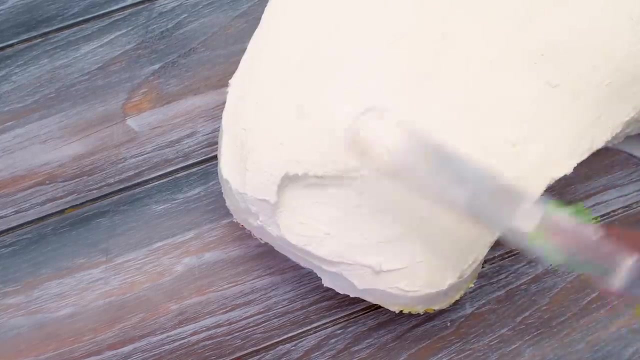 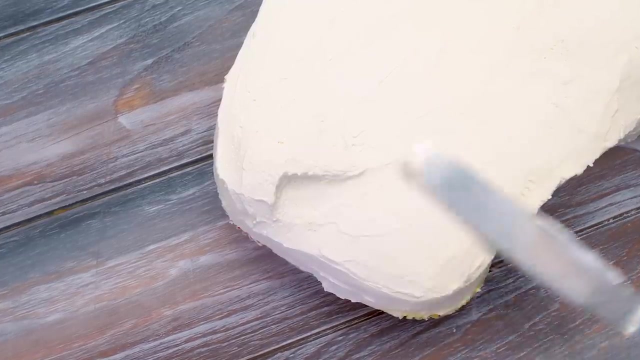 And this will help us make a cheek for our unicorn. Here we go. I think it looks beautiful and pretty realistic, Do you agree, guys? And let's not forget about the nose This way. All right, Beautiful, Our unicorn is finally taking its shape. 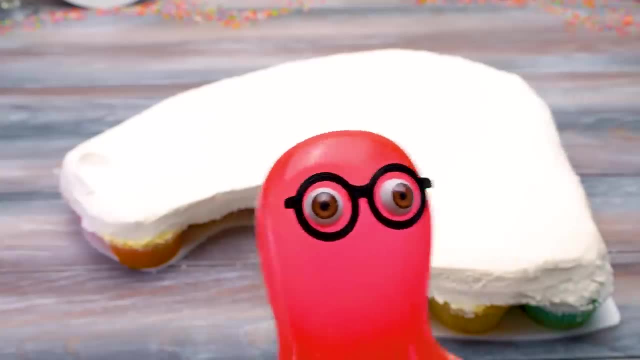 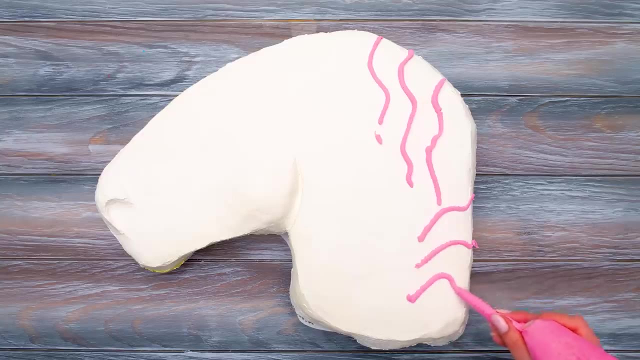 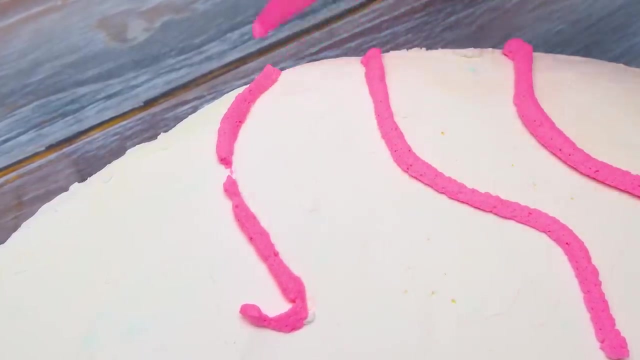 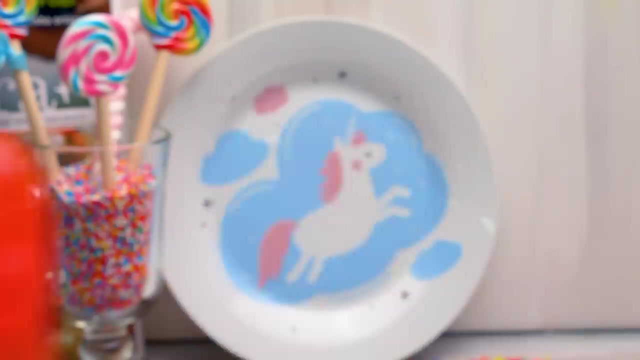 Sue, it still doesn't look like a unicorn to me. That's because we still need to add more details. Our beautiful unicorn will have a fancy colorful mane. I decided to start with pink. Carefully, don't brush, Sue. I've been thinking: why don't unicorns count as a wonder of the world? 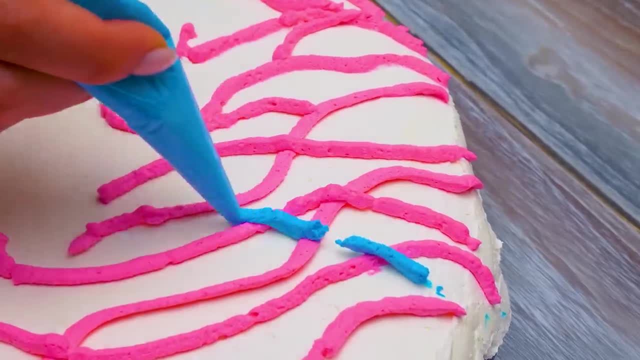 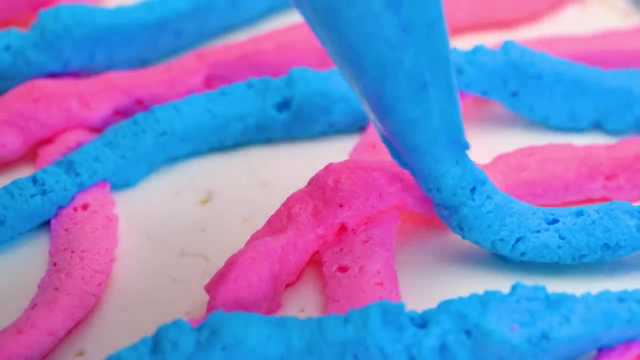 I mean, they're so sweet and awesome. That's a good question. Unicorns deserve their place in the world's wonders list. I know that there are several lists of the wonders of the world. The oldest one was made by ancient Greeks. 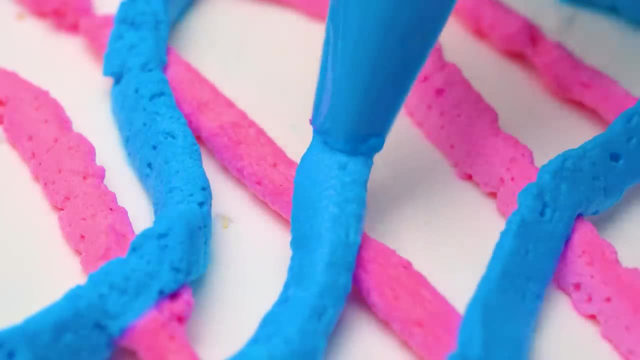 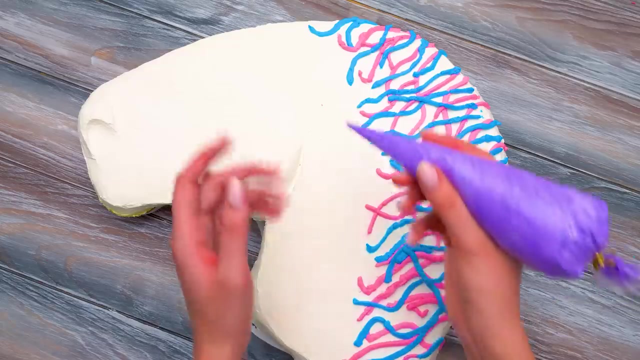 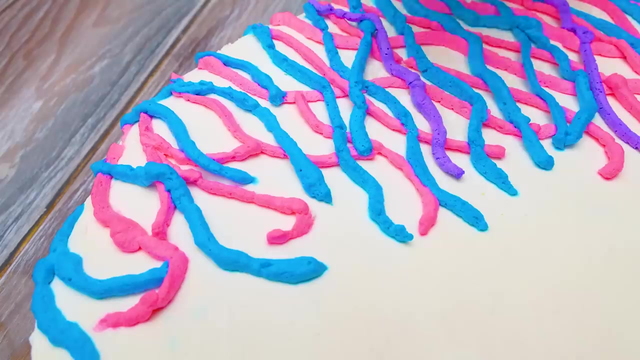 Any ideas what it contains? Sammy? Let me guess Olives, then laffetta cheese. Sammy, those are stereotypes about Greece. That list mainly has architectural items actually. Huh, I just opened that list on Wikipedia. The only exception is the Hanging Gardens of Babylon. 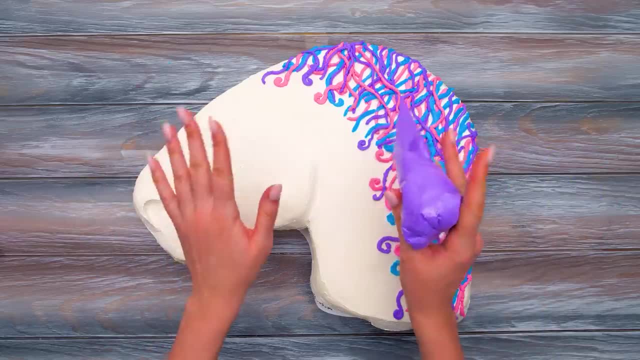 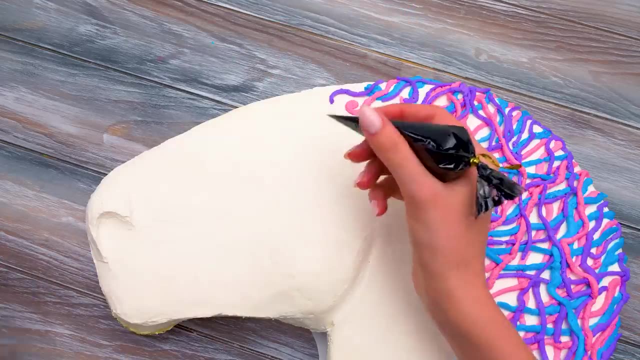 Why exception? By the way, I can name all the ancient wonders of the world. Sounds ambitious, Bring it Susie. The Great Pyramid of Giza, The Hanging Gardens, The Statue of Zeus at Olympia, The Temple of Artemis. 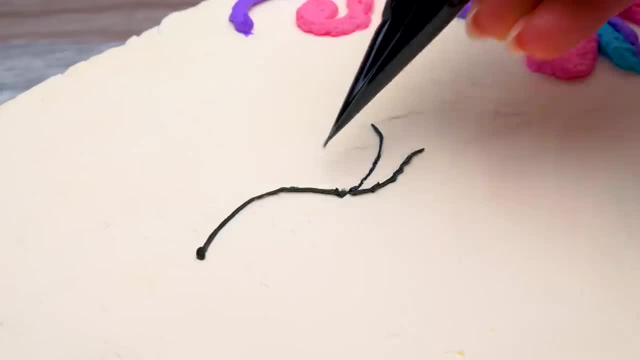 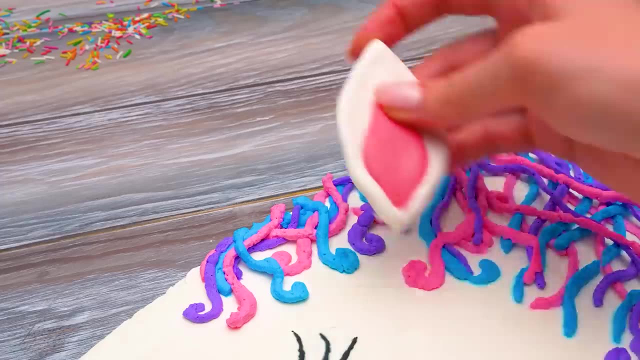 The Mausoleum at Halicarnassus, The Colossus of Rhodes And the Lighthouse of Alexandria. Not bad, not bad. How's our unicorn cake? I've just made an ear for it. Look how great it is.